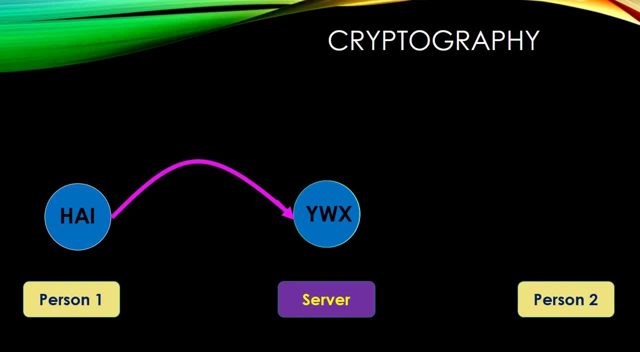 And it will be saved as something which we cannot able to decrypt. So person 1 is sending hi and at the server it is stored as something like ywx, And this process is called encryption. Once it is saved as ywx, then person 2 cannot be able to understand what is ywx, So he wants to read it as the same hi. 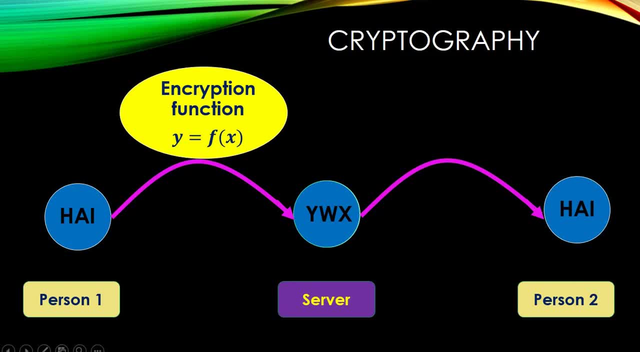 And this can be done by inverse function of encryption. That is nothing but decryption function, And this can be done by inverse function of encryption. That is nothing but decryption function. And how this is possible we will see with a simple example And how matrices are helpful in cryptography. 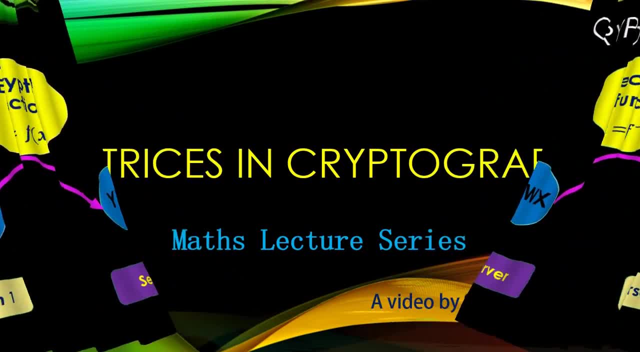 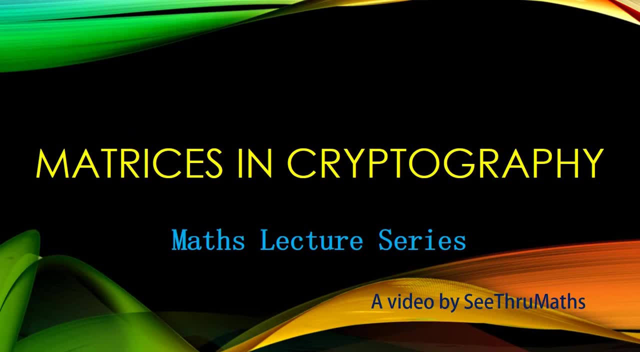 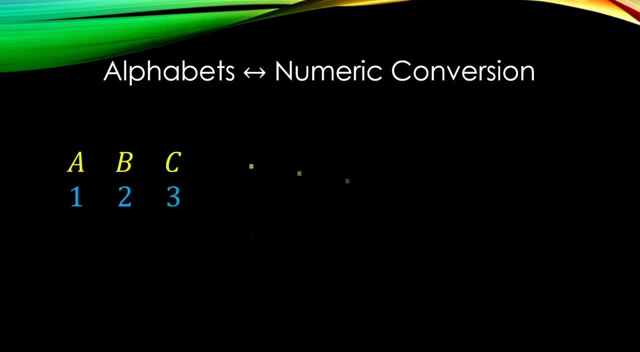 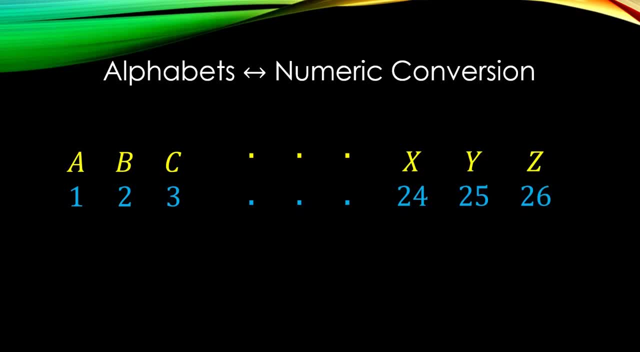 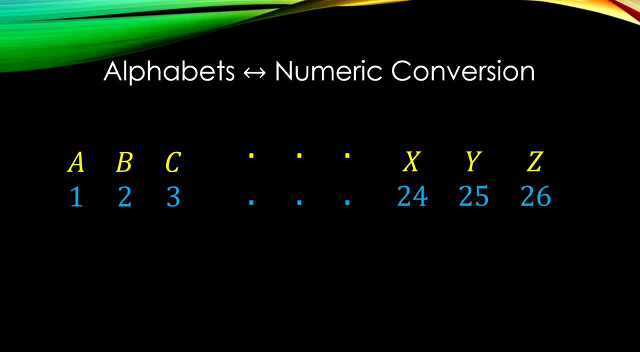 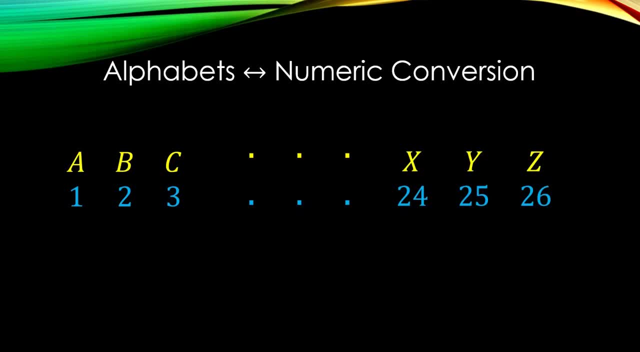 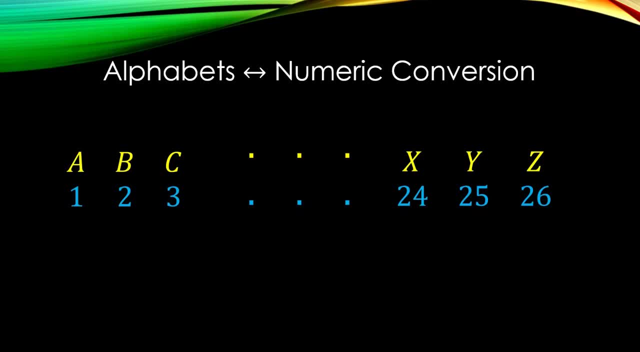 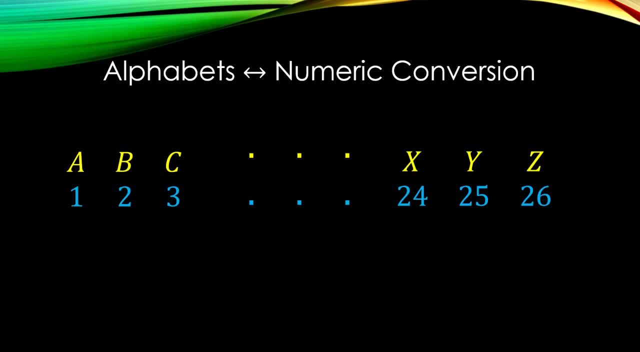 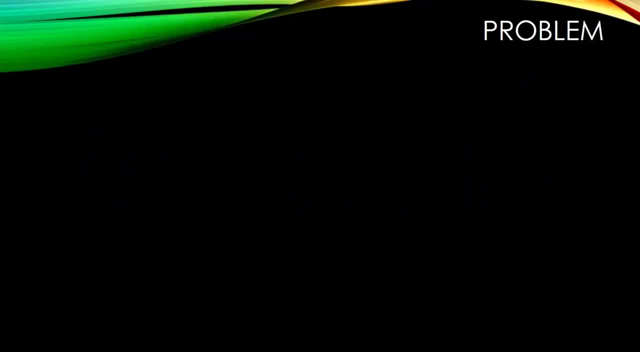 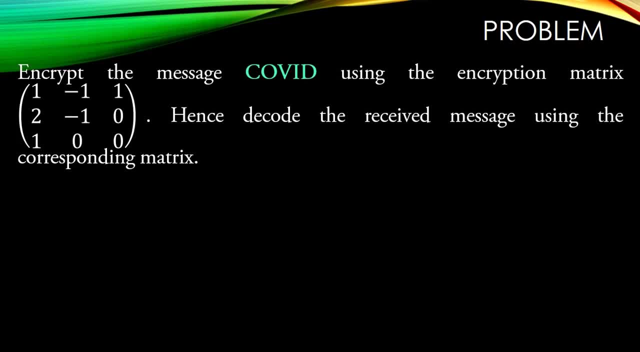 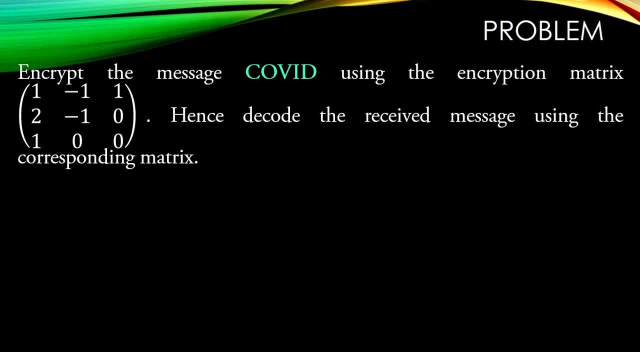 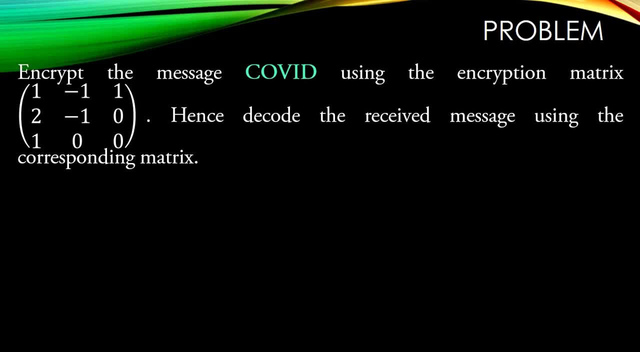 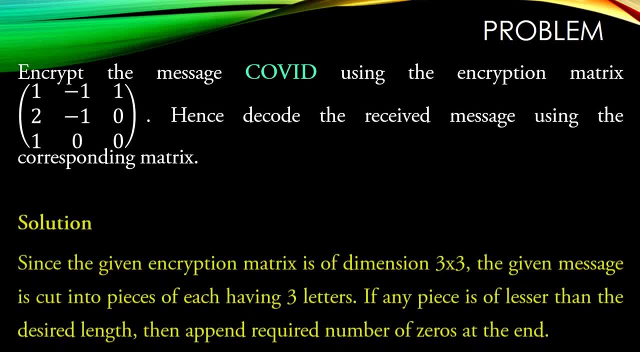 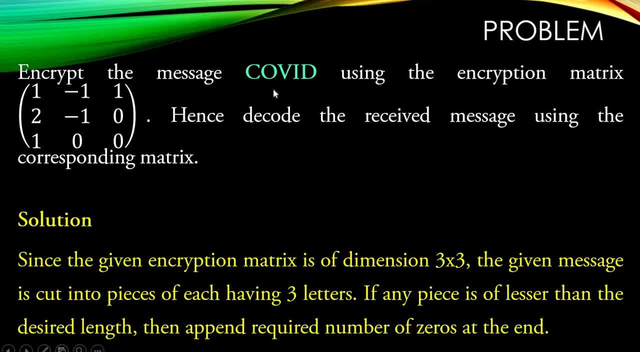 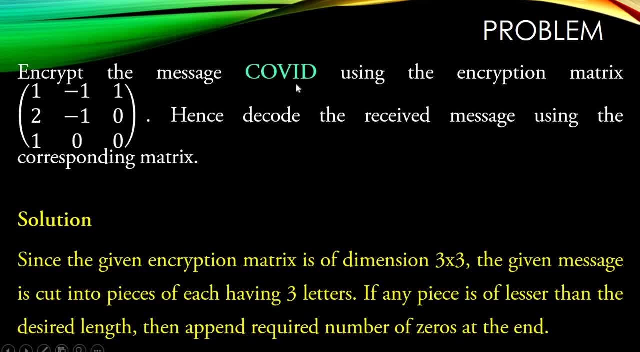 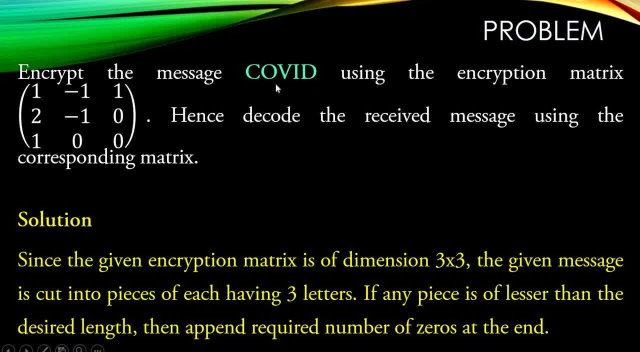 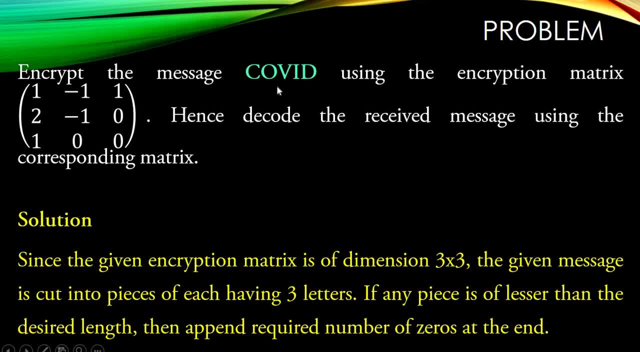 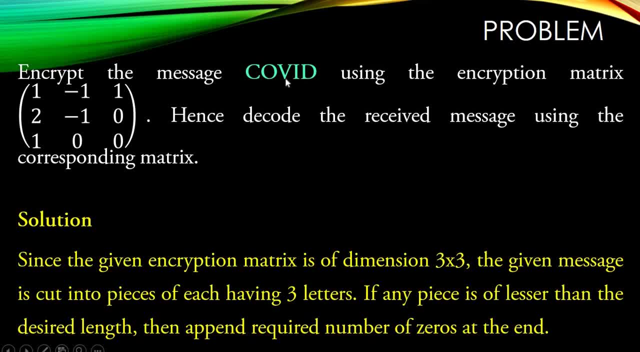 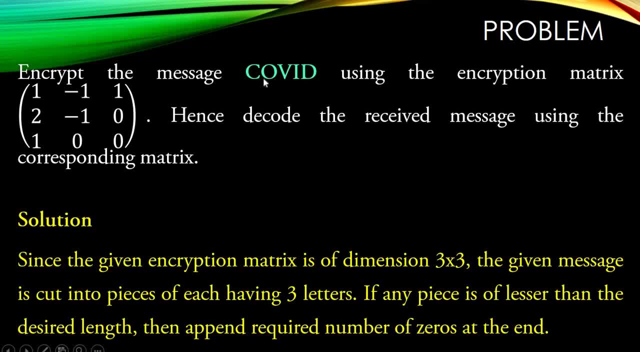 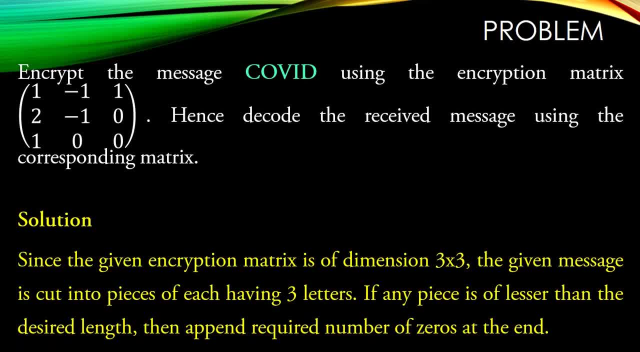 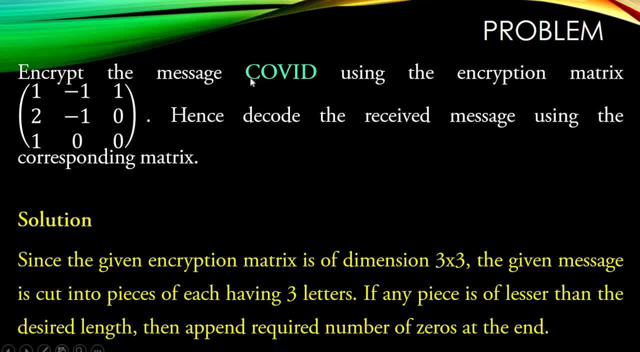 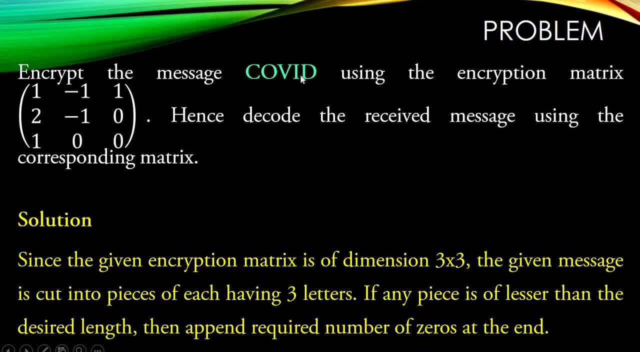 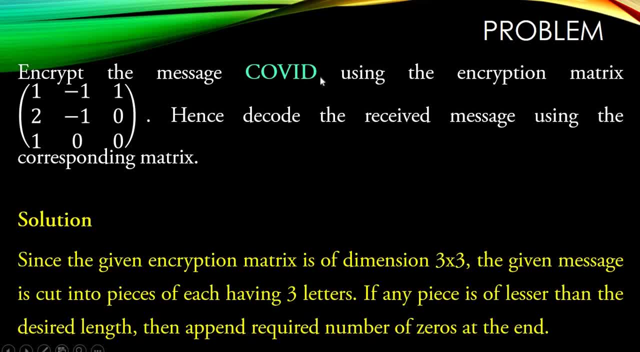 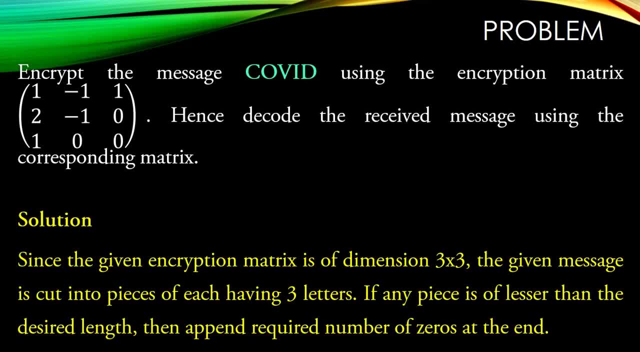 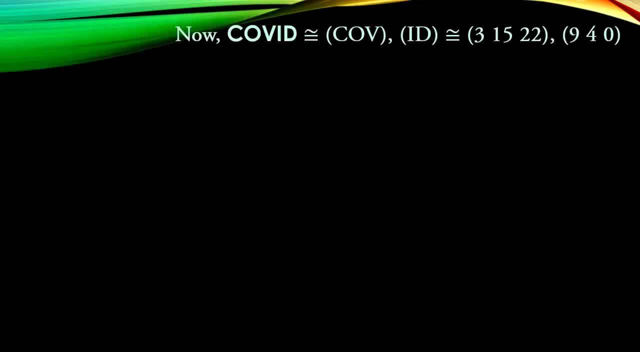 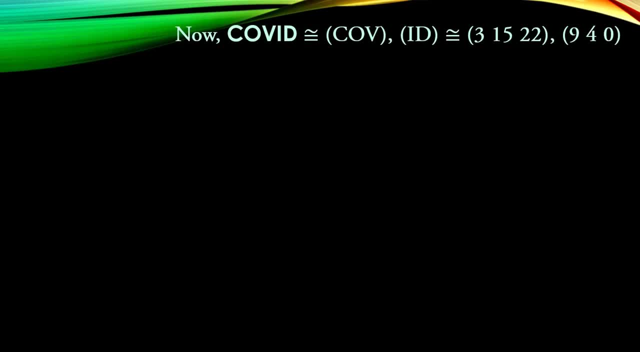 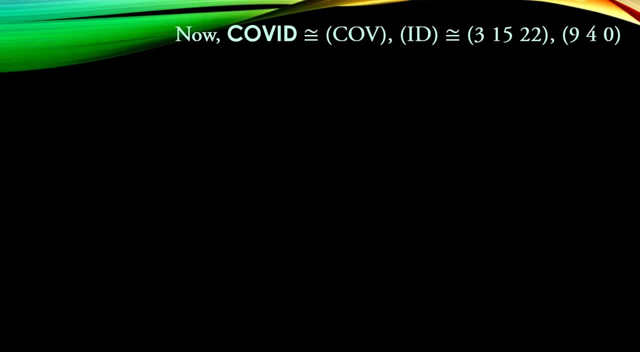 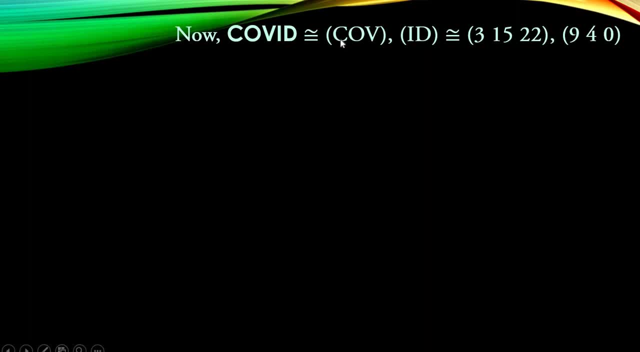 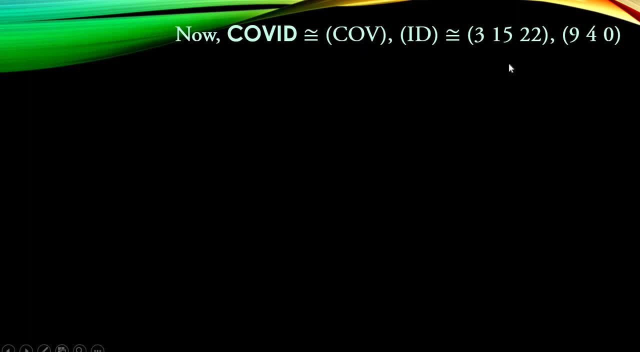 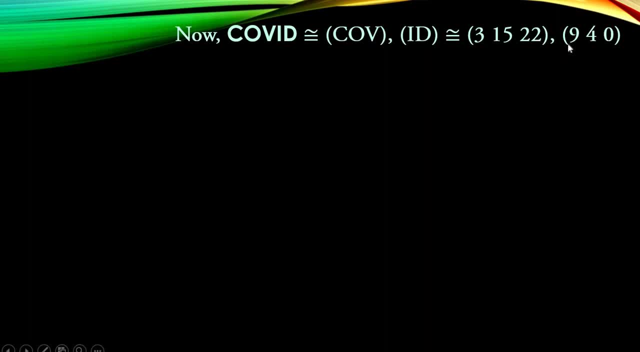 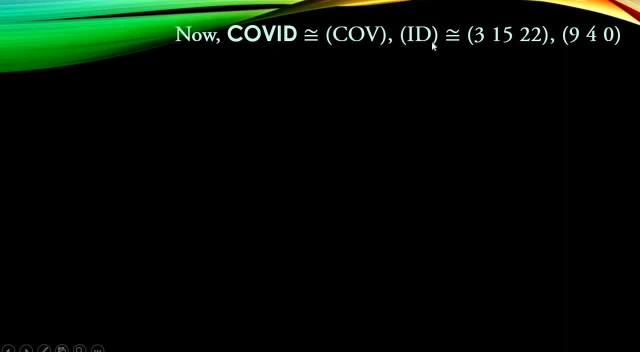 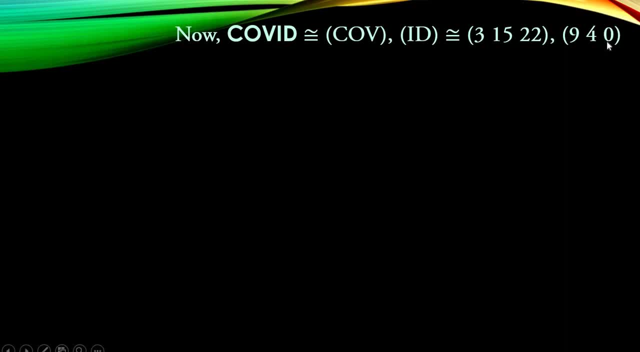 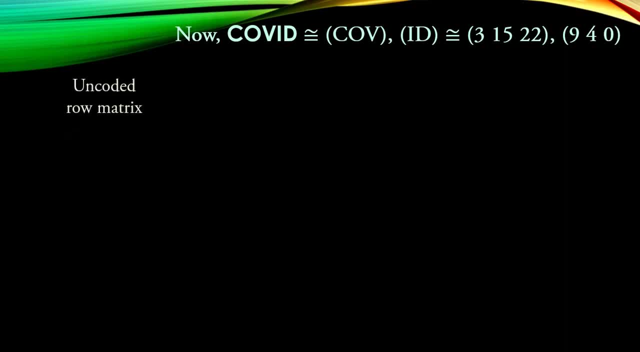 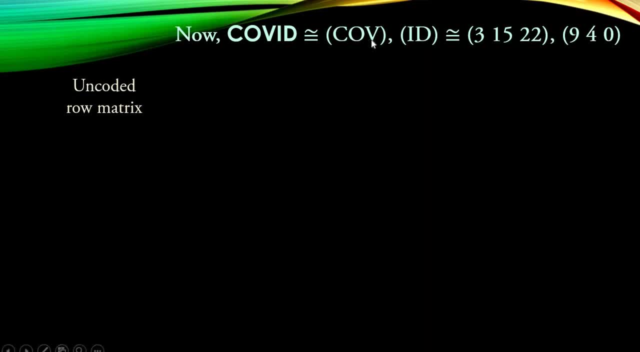 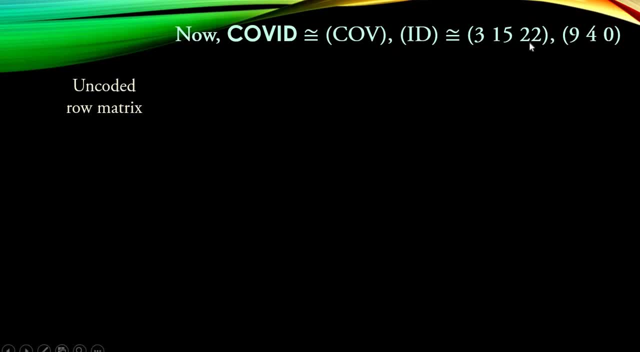 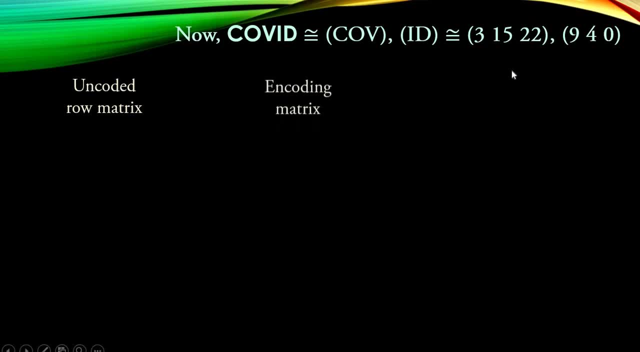 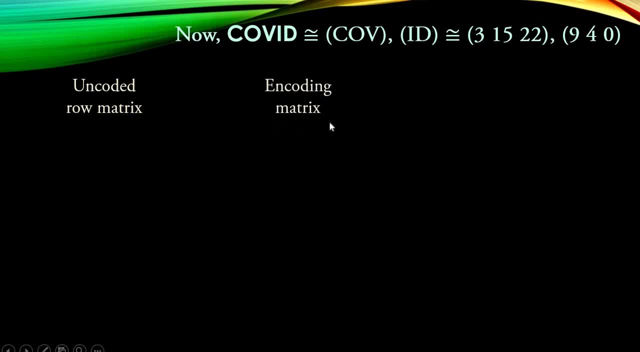 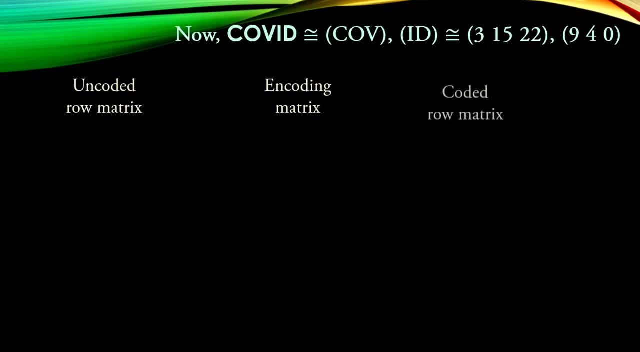 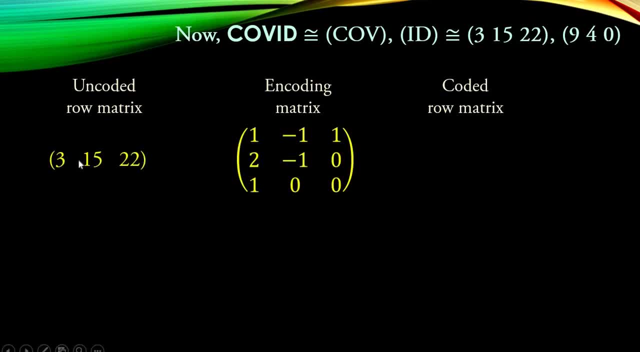 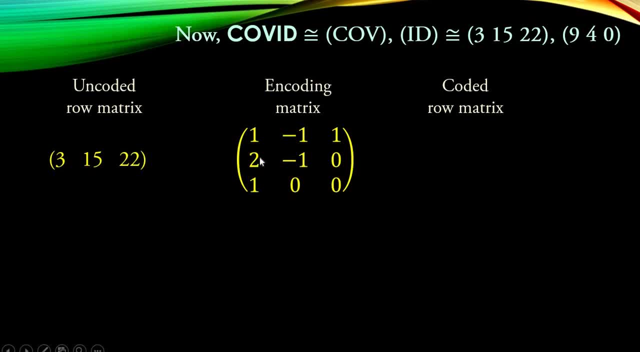 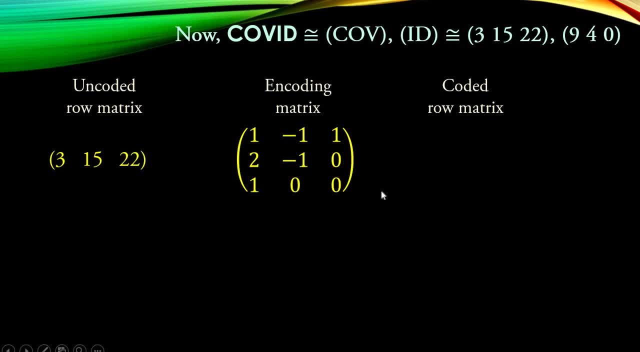 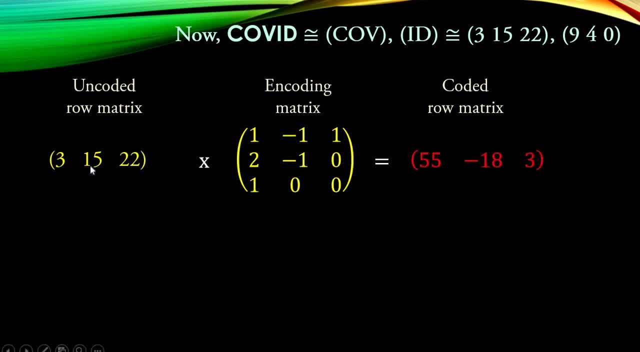 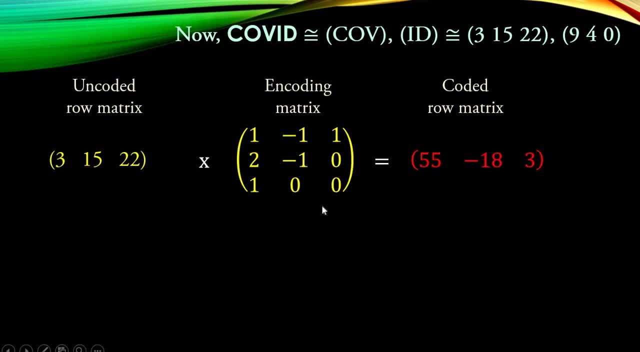 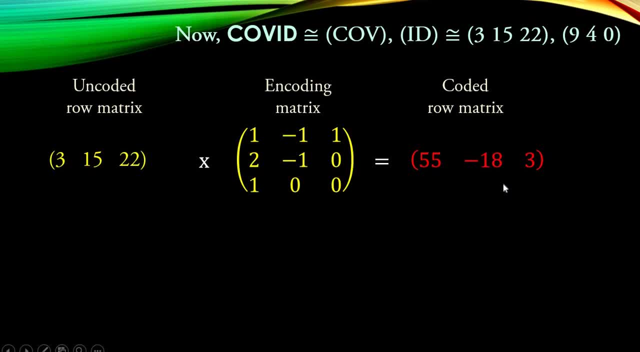 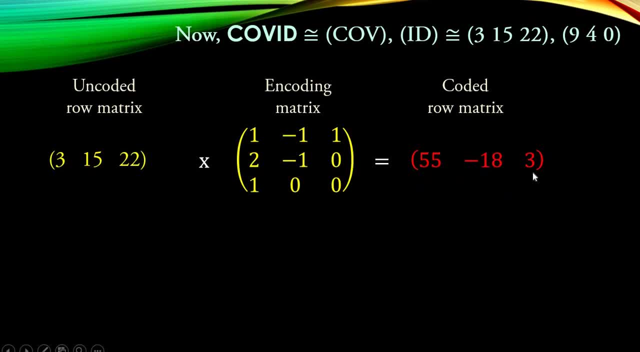 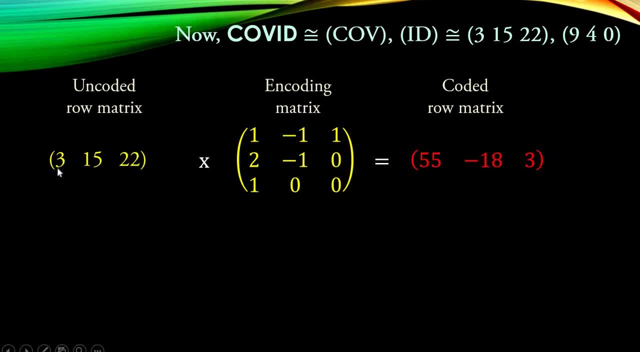 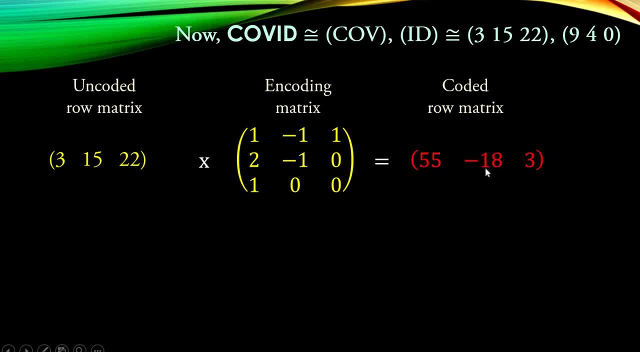 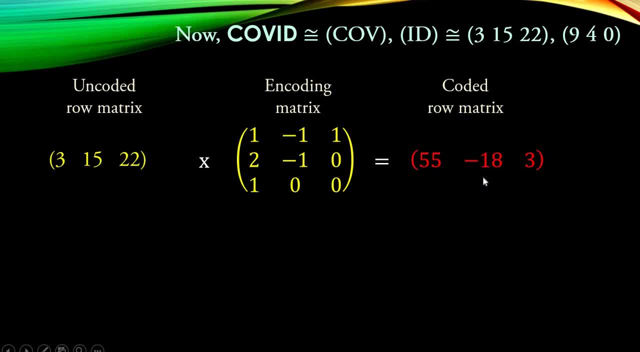 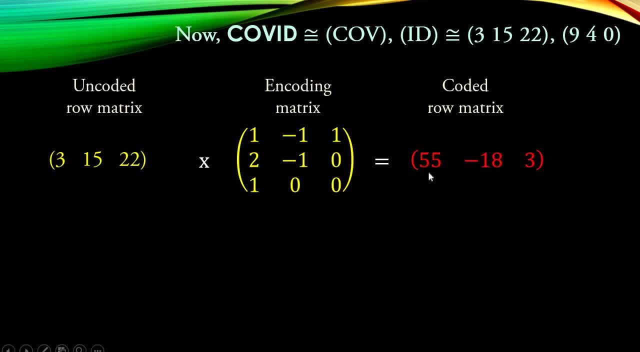 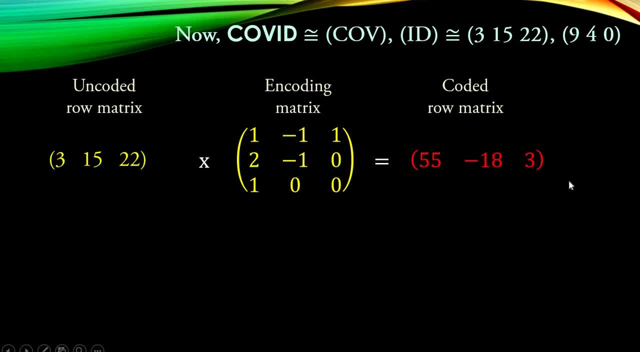 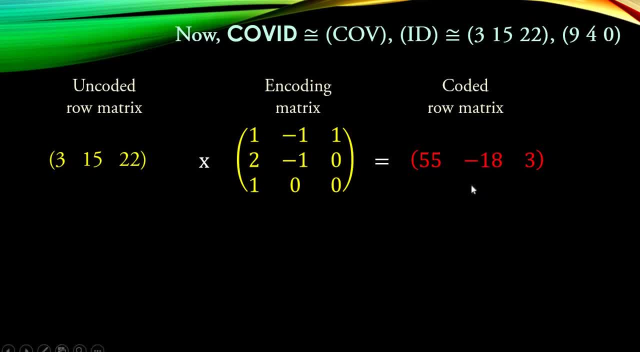 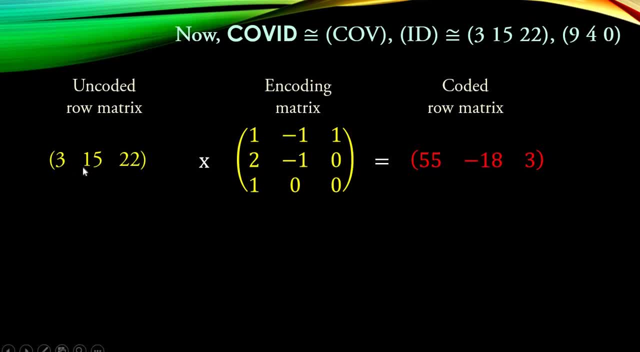 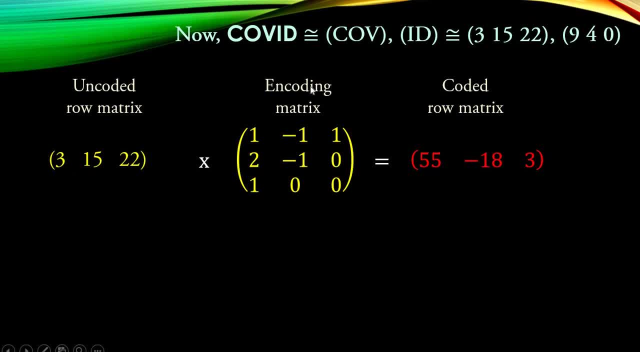 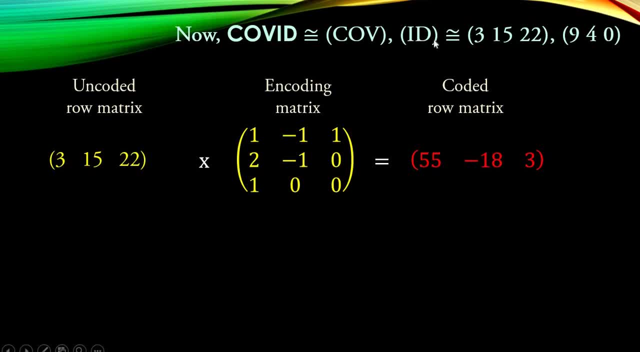 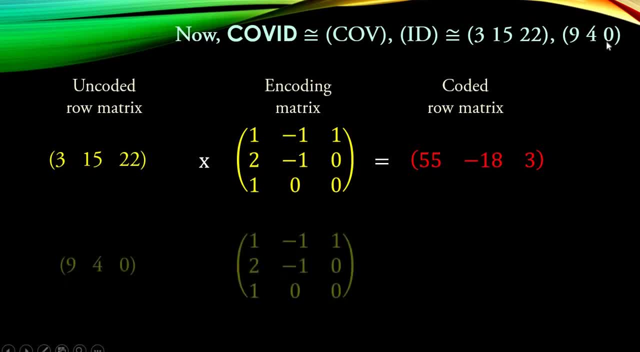 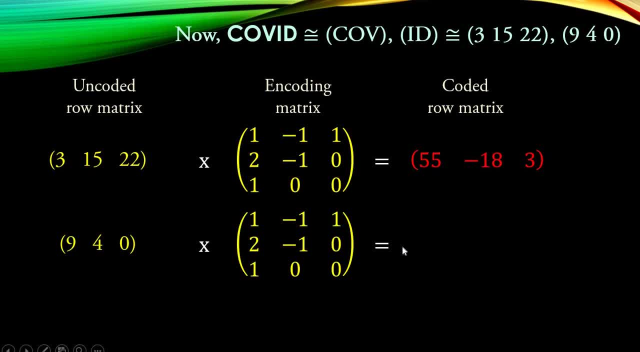 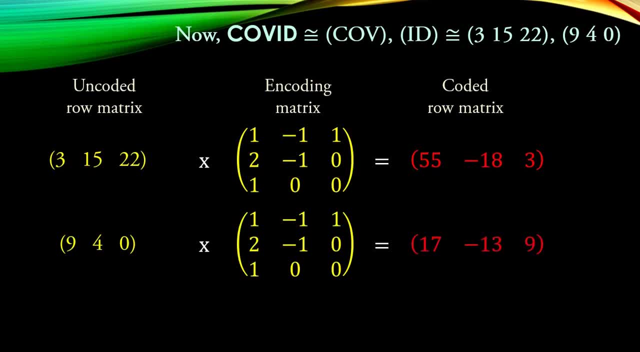 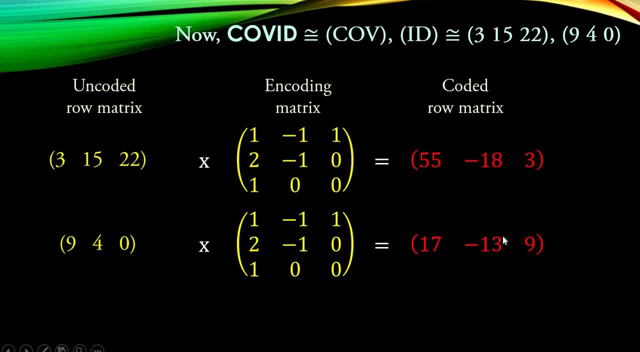 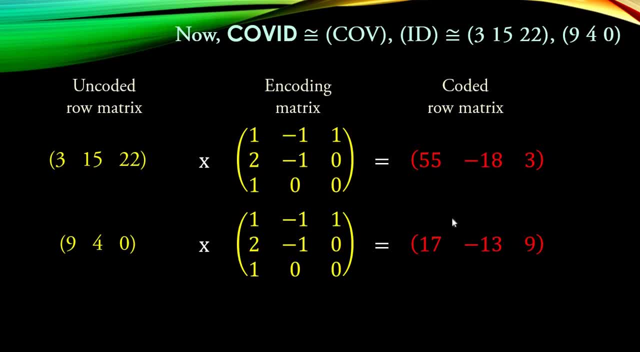 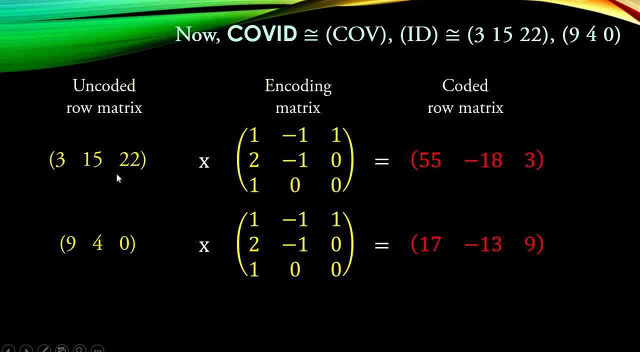 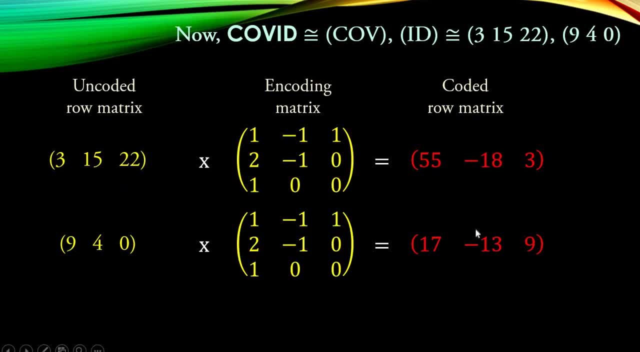 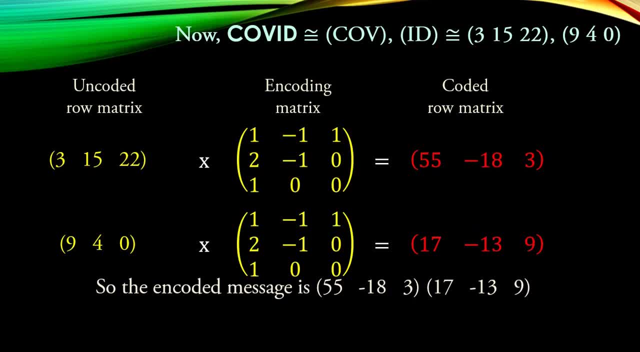 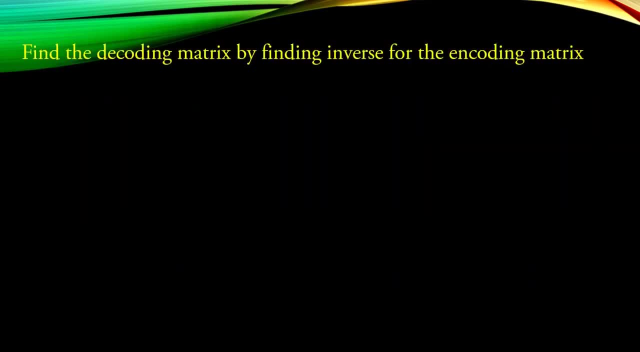 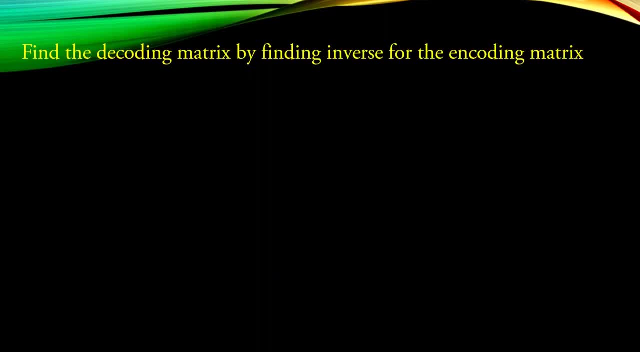 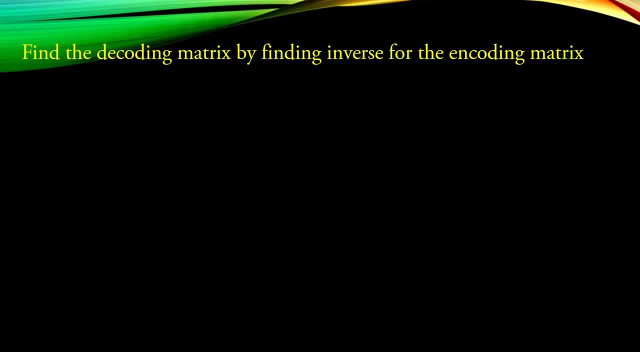 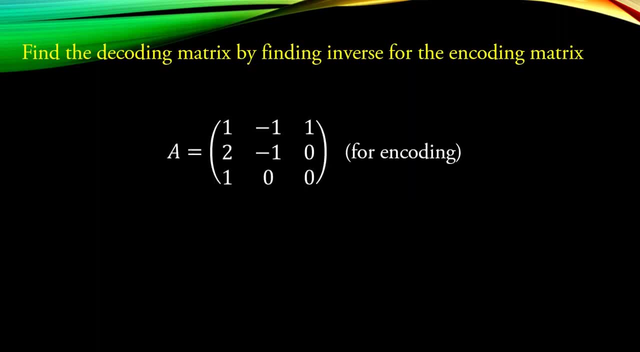 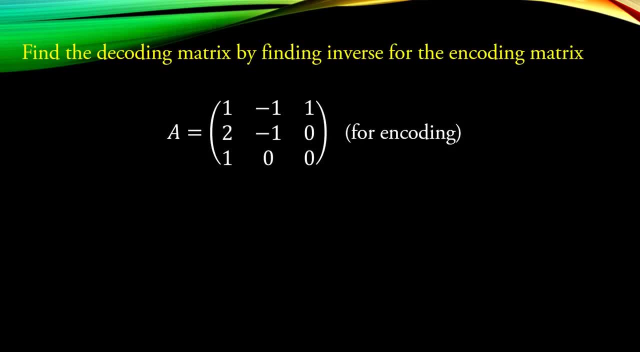 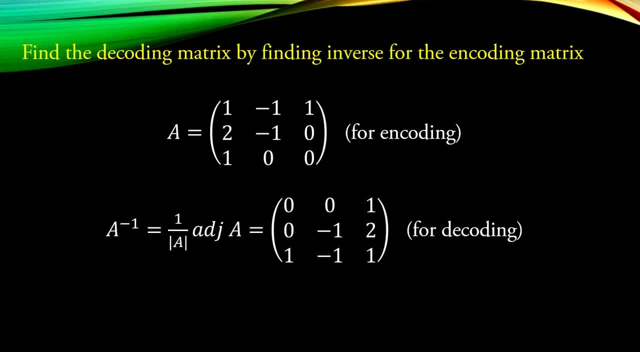 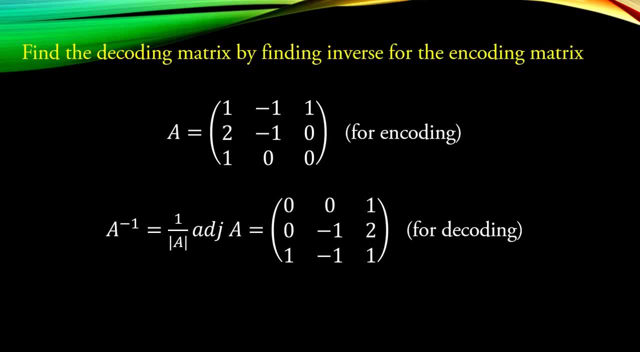 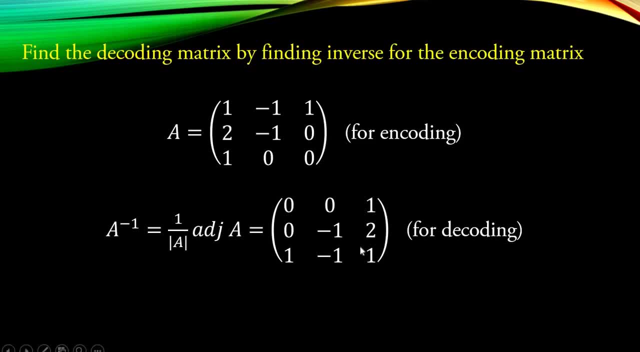 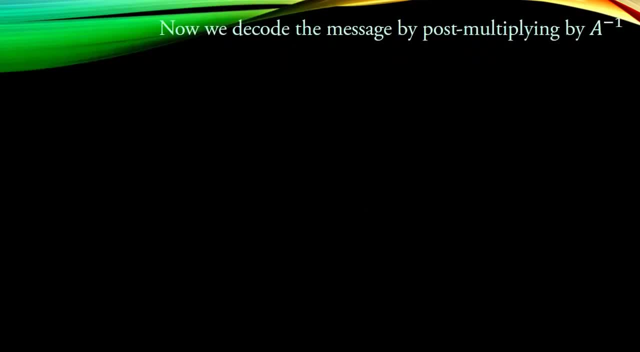 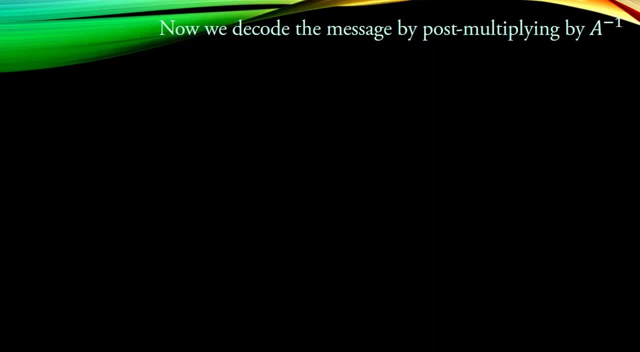 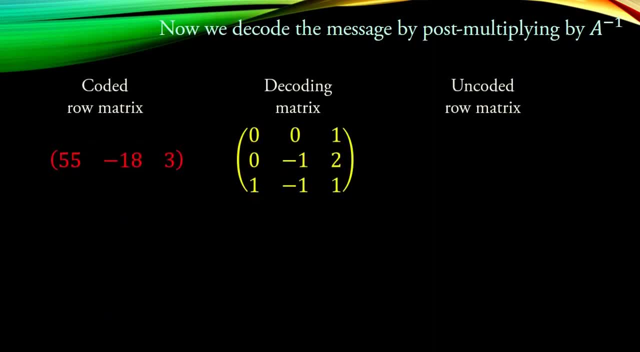 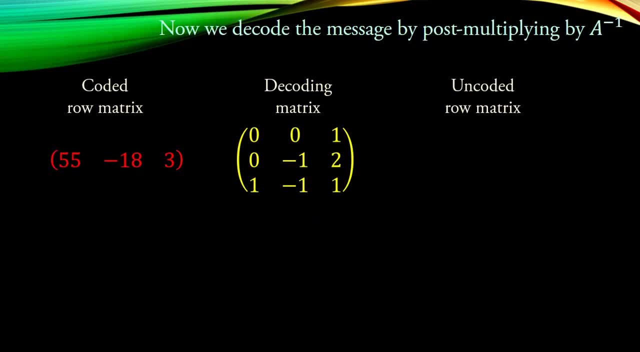 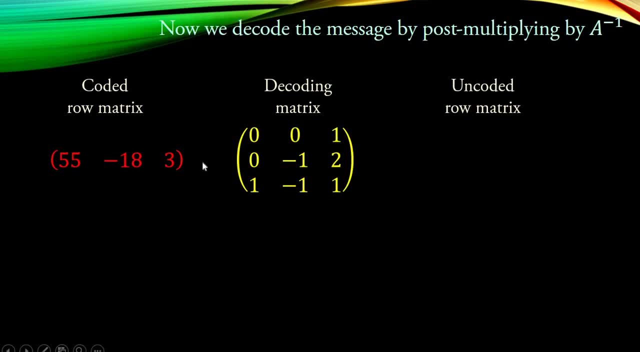 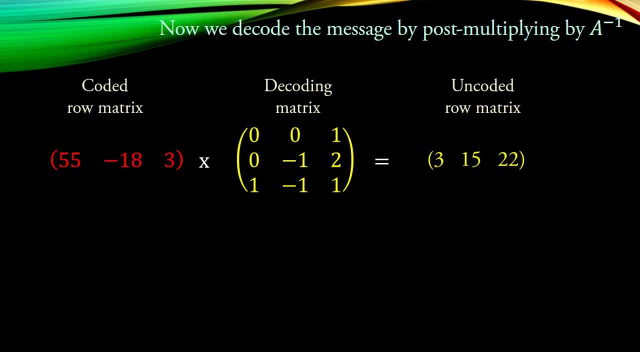 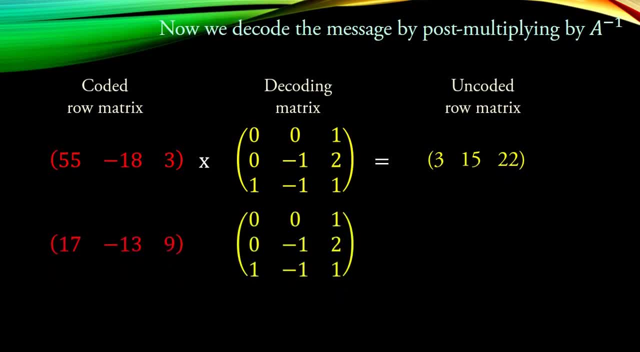 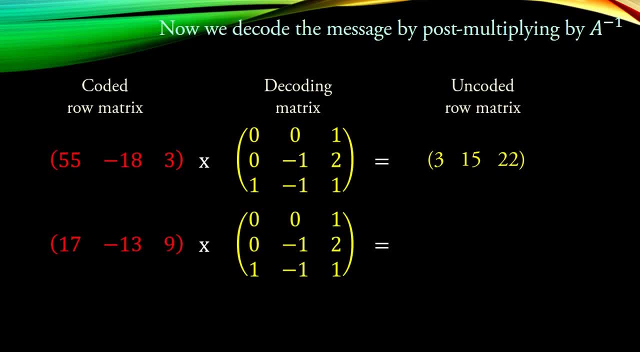 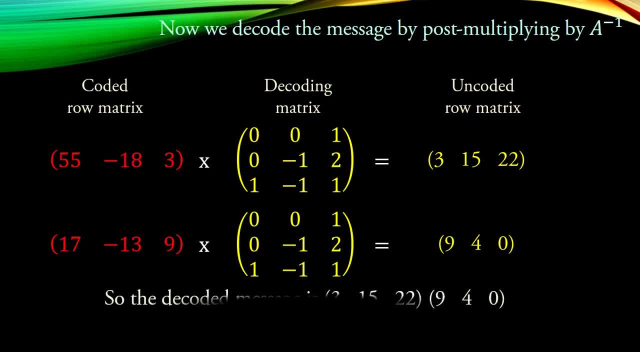 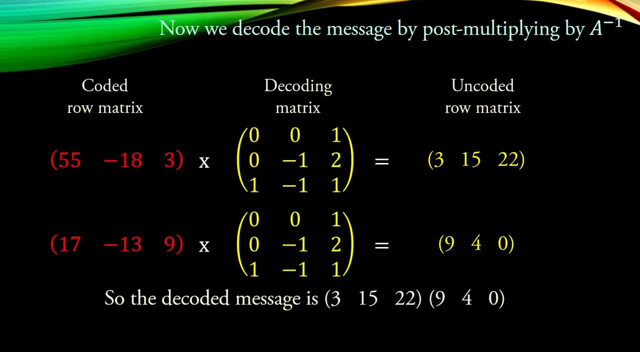 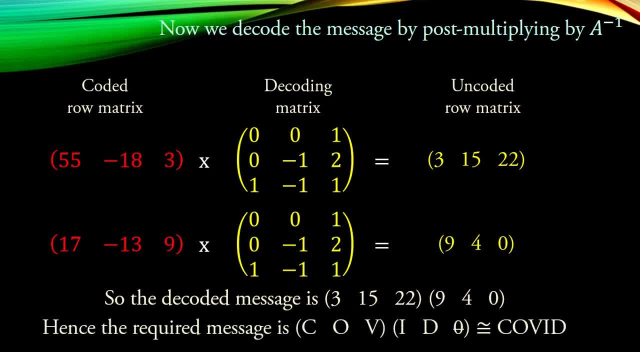 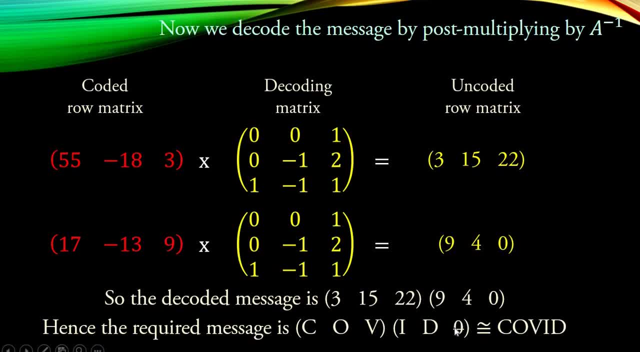 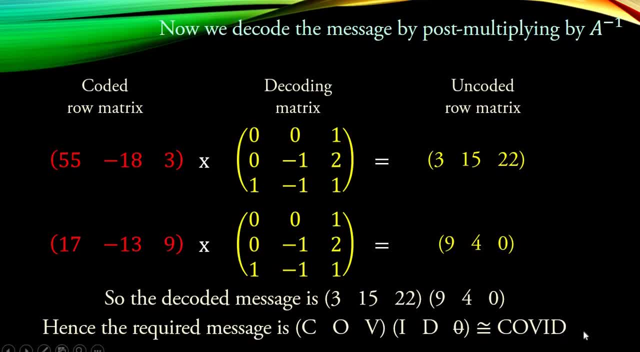 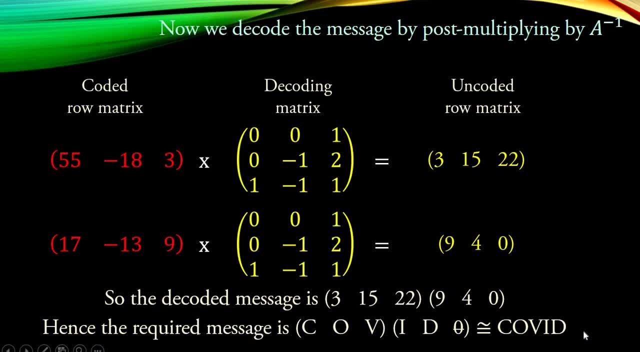 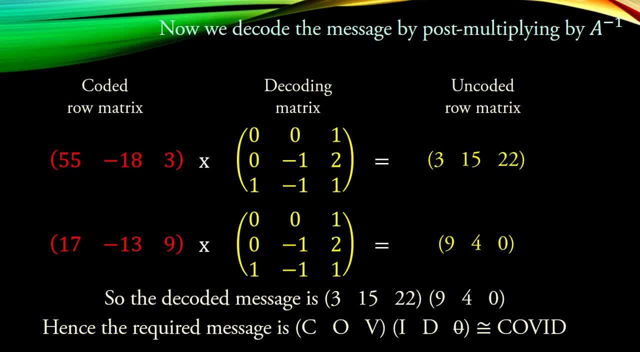 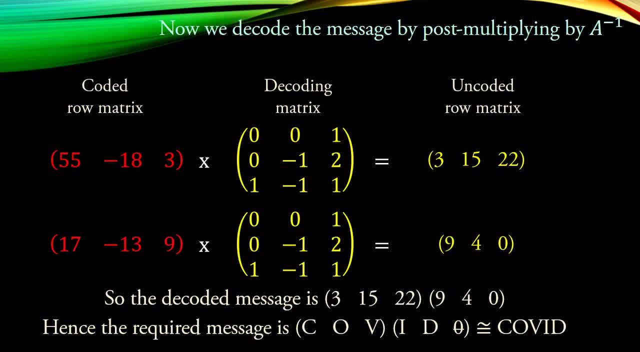 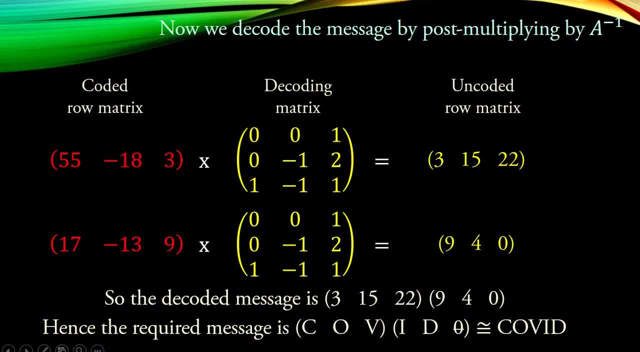 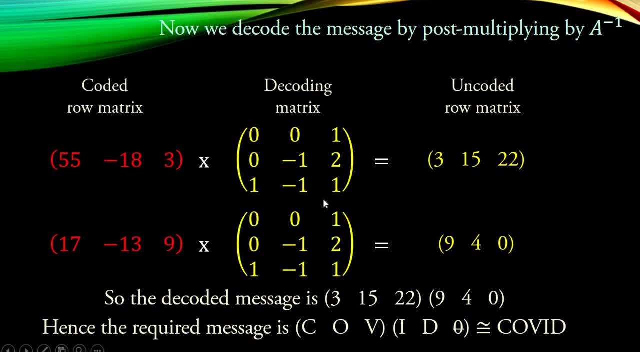 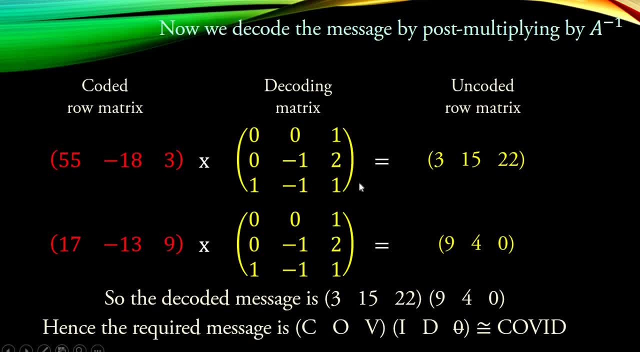 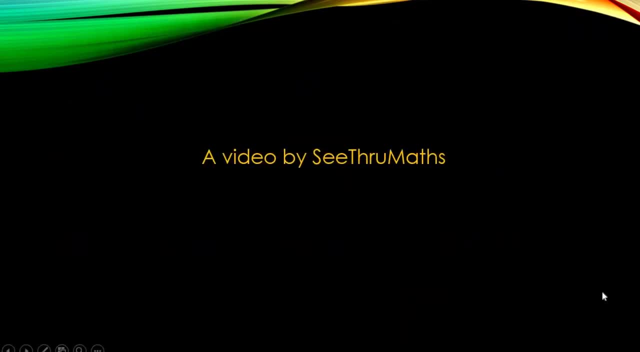 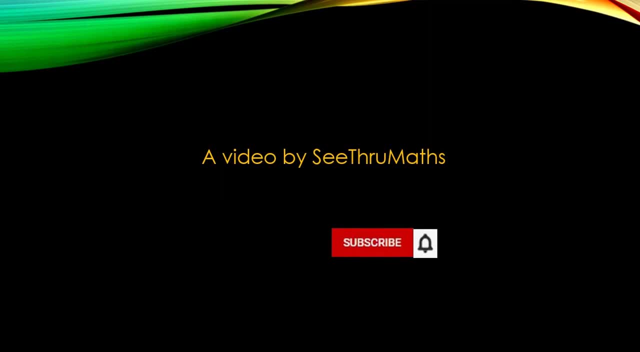 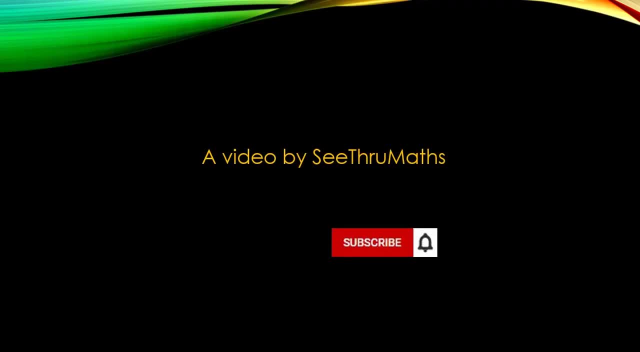 So A, B, C, D, and these are the alphabets named as 1,, 2,, 3 and so on.